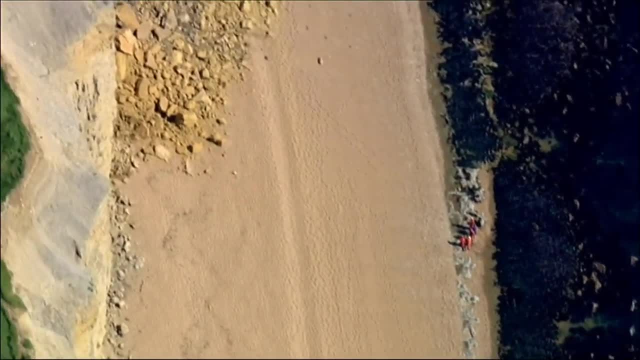 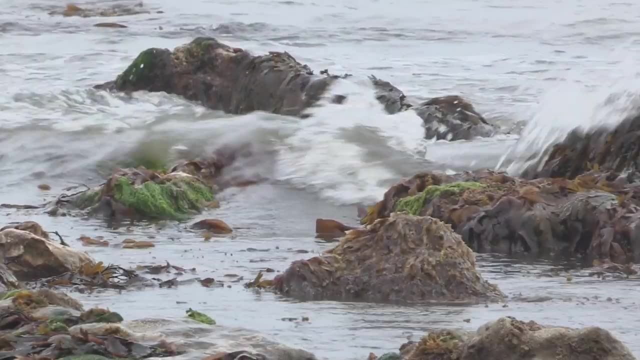 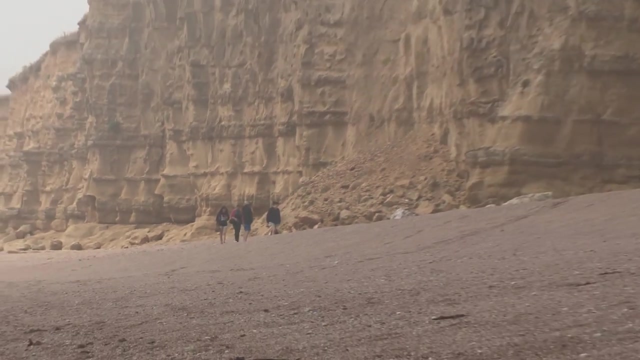 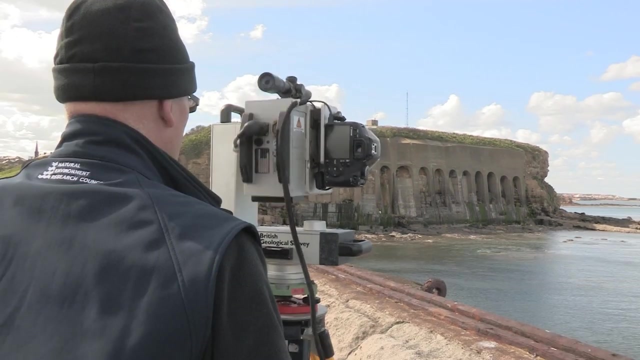 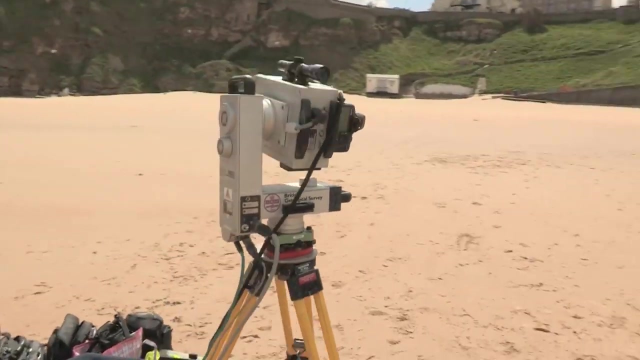 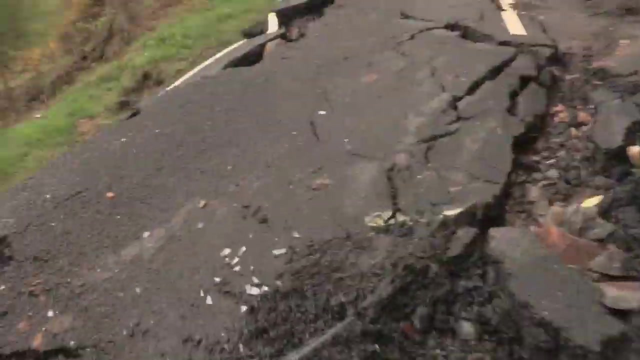 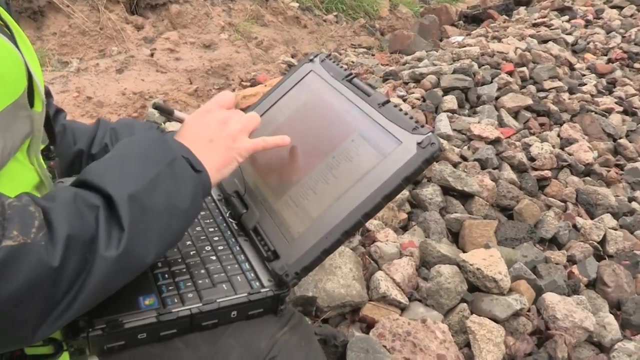 I'm going. So if we can't stop them, what can we do? The answer at the British Geological Survey is: plenty Music. This is the work of the landslide team at the BGS: Cutting edge technology for cutting edge research, Any kind of detailed measurement- this instrument is ideal. 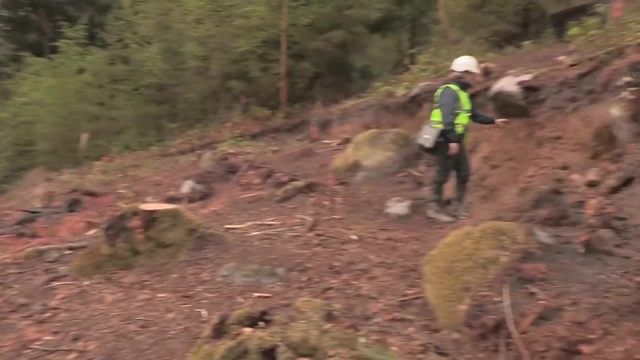 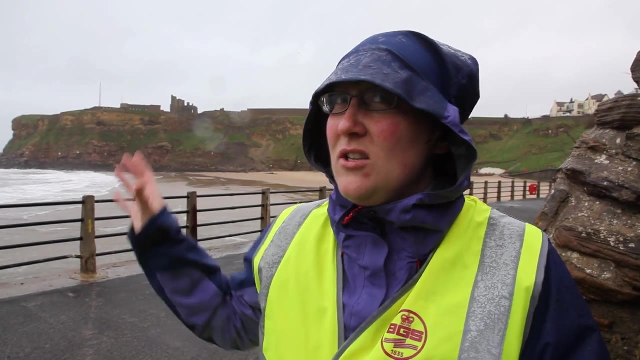 Learning more about how landslides happen. What we want to do when we're in the field is we want to record the details And seasonal weather again and you can see really why this is such a dynamic environment and why we get these events happening. 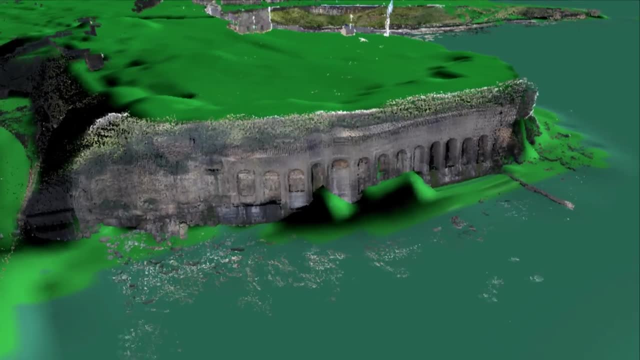 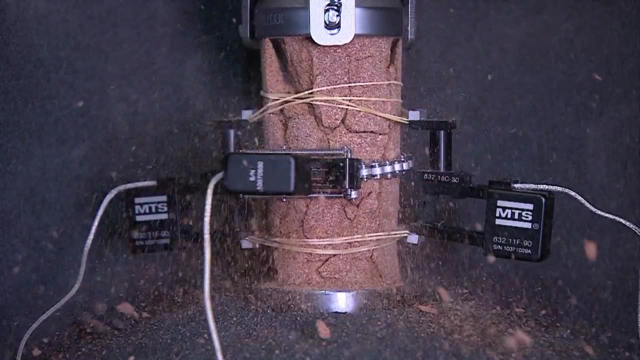 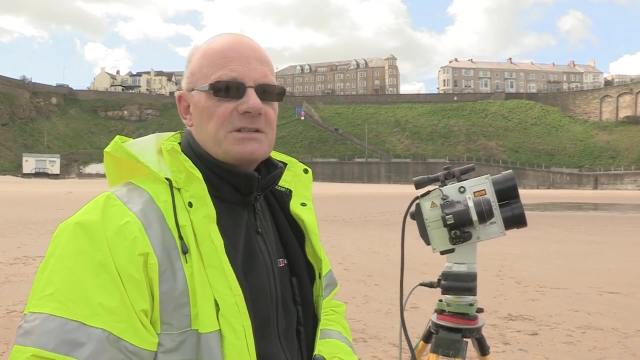 Giving all of us more information. We help people Where we have information we make it available, Making all our lives safer. Studying the processes that lead to these geohazards so that we can try and avoid them in the future. Music. 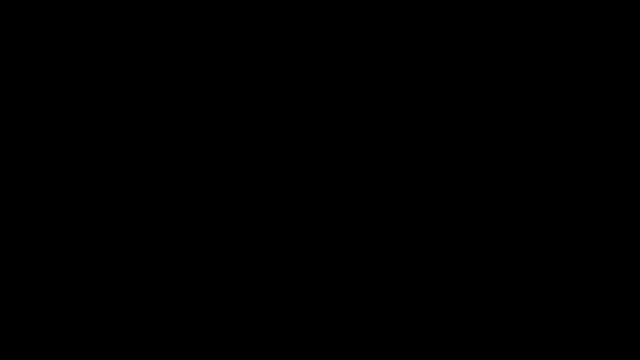 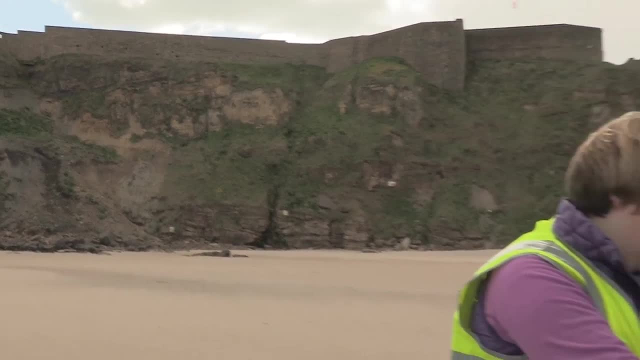 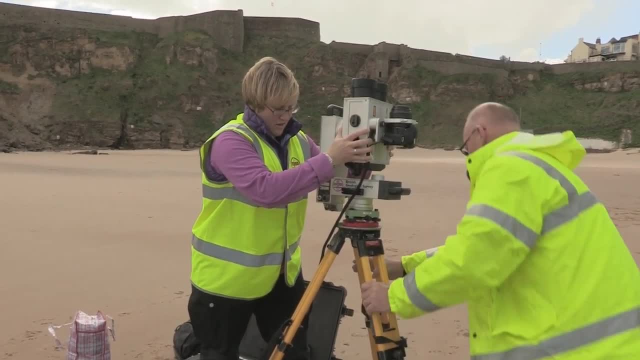 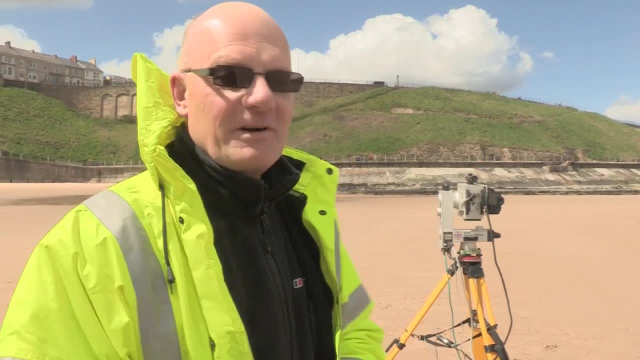 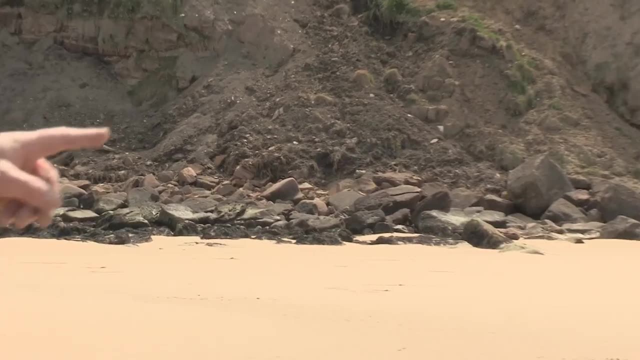 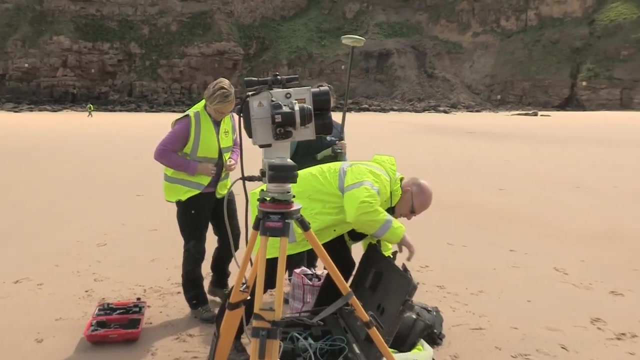 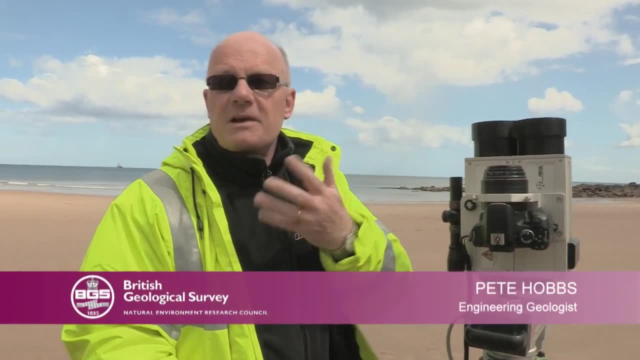 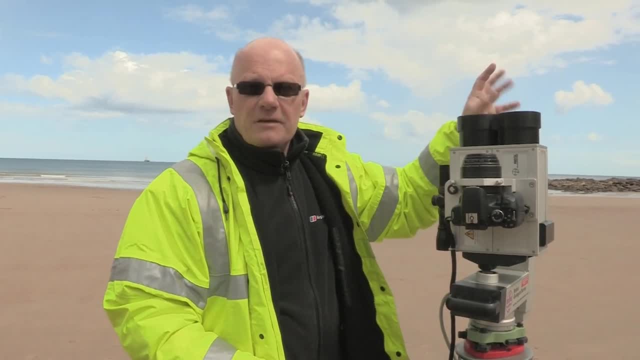 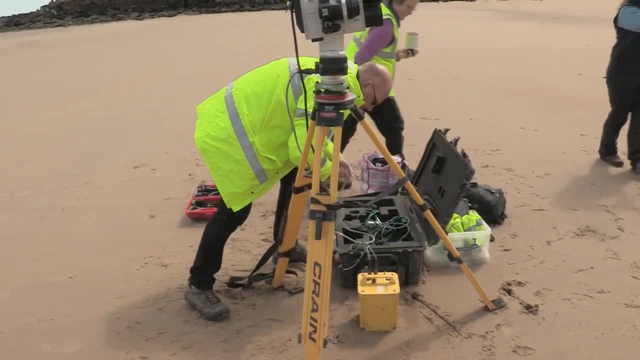 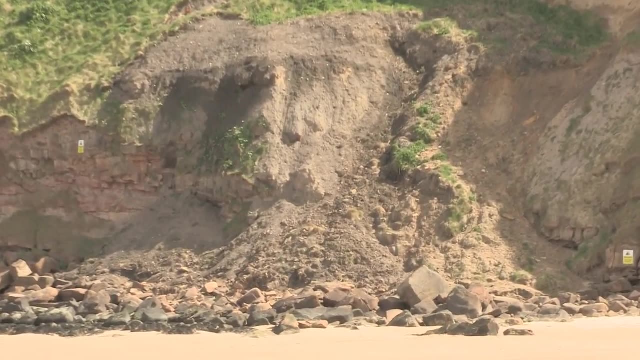 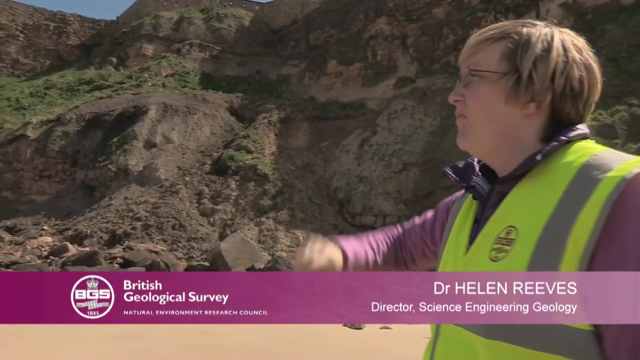 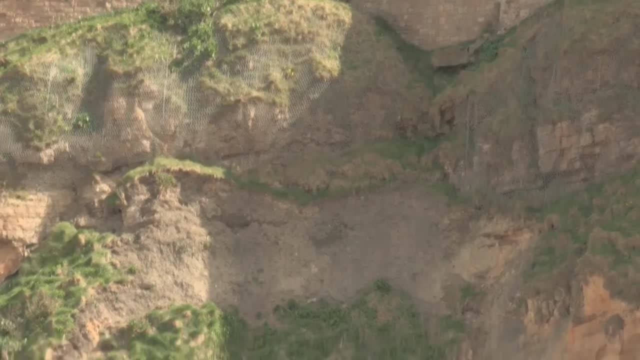 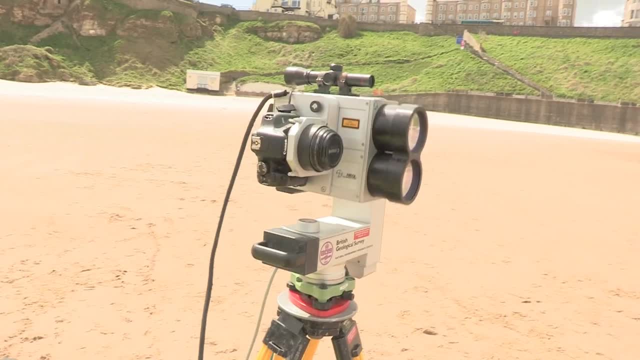 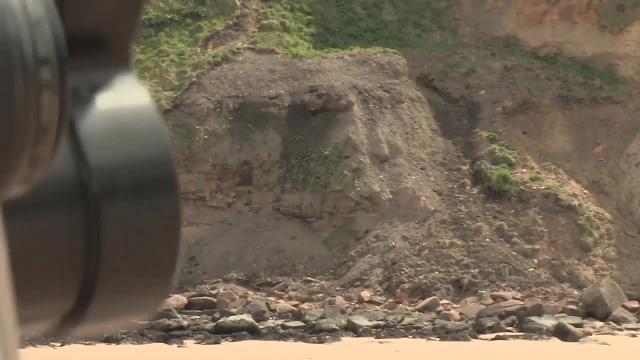 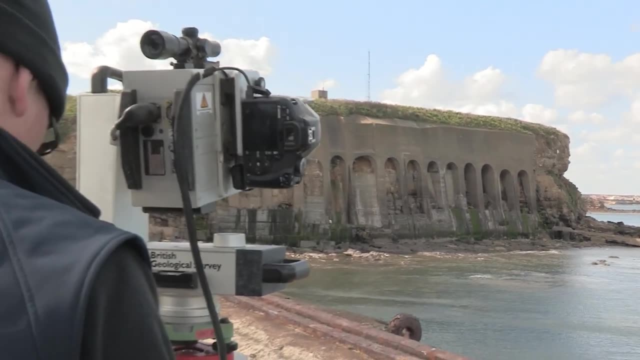 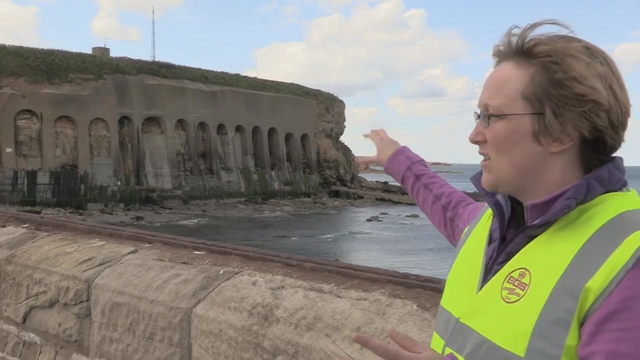 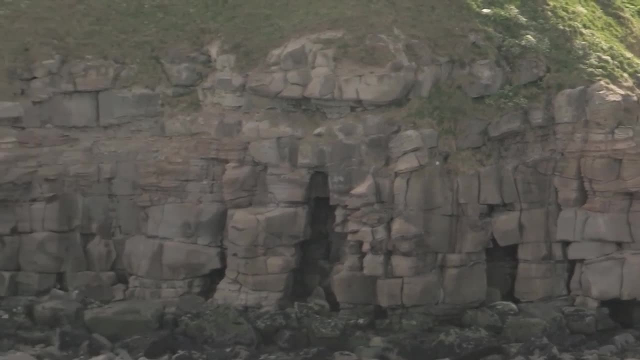 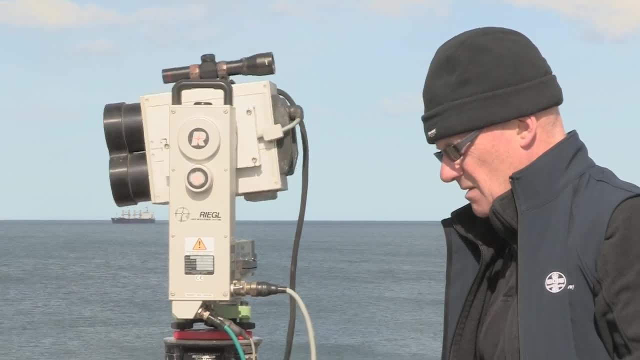 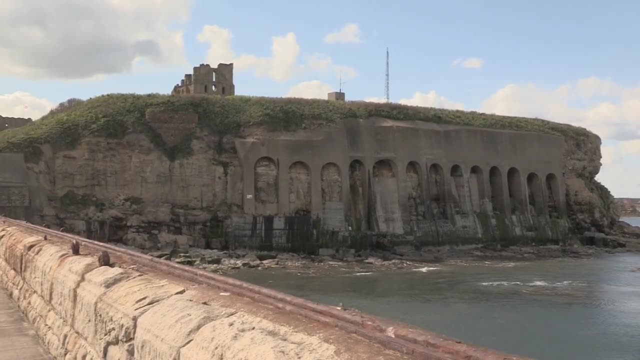 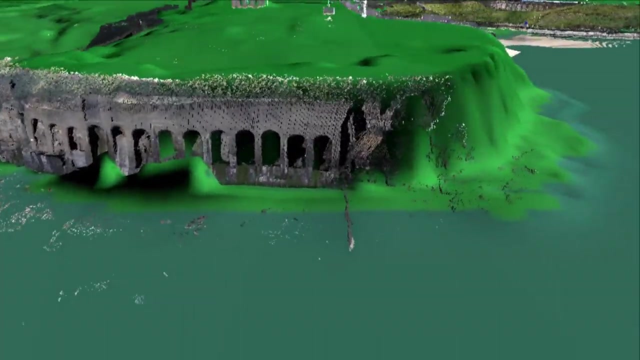 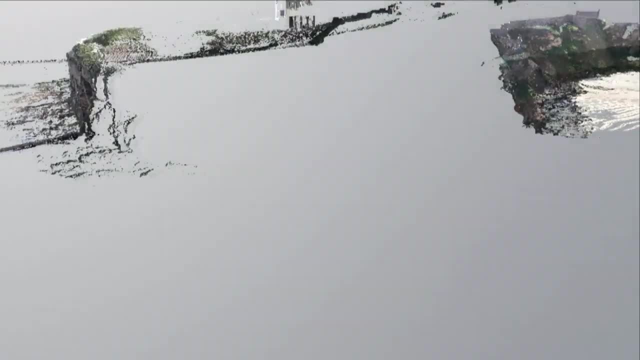 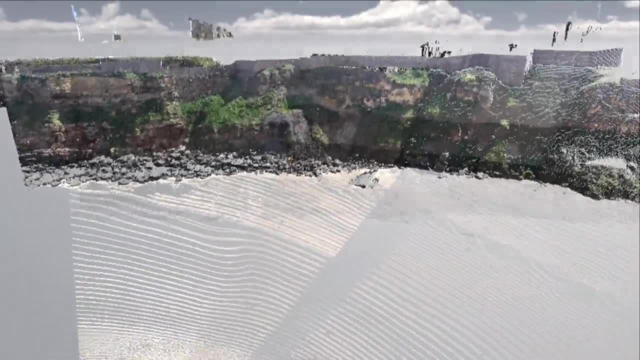 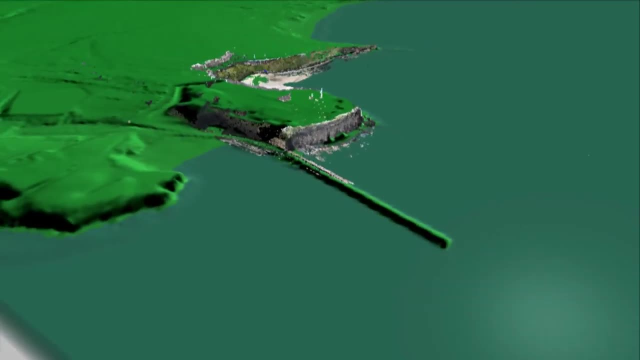 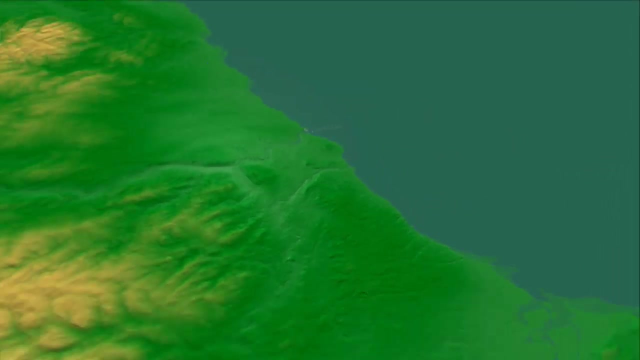 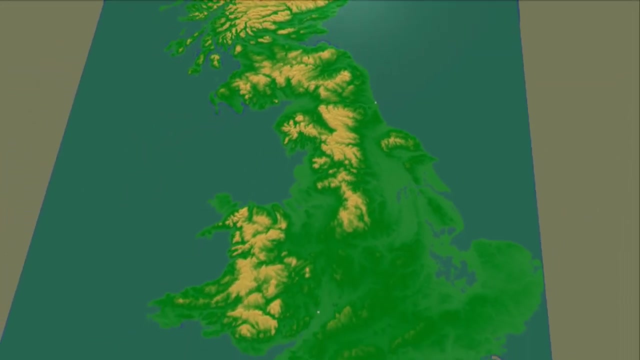 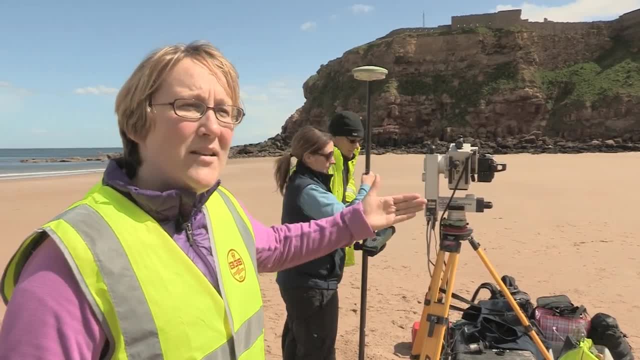 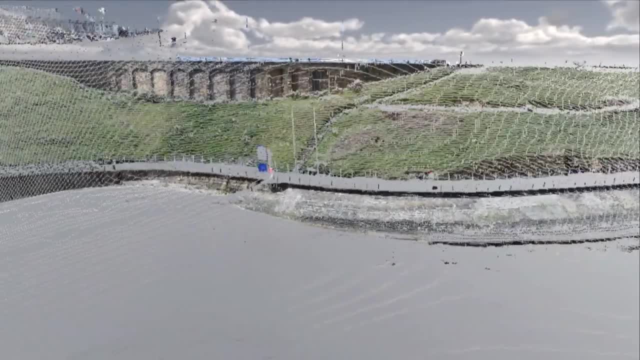 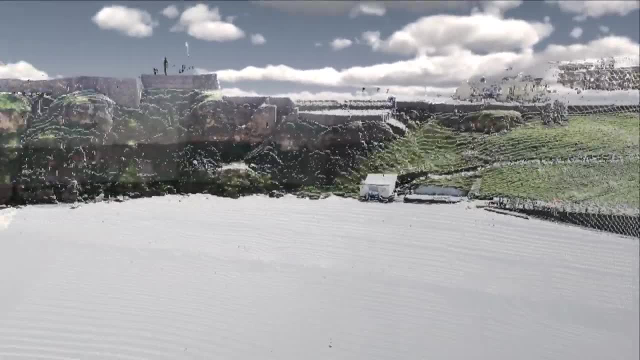 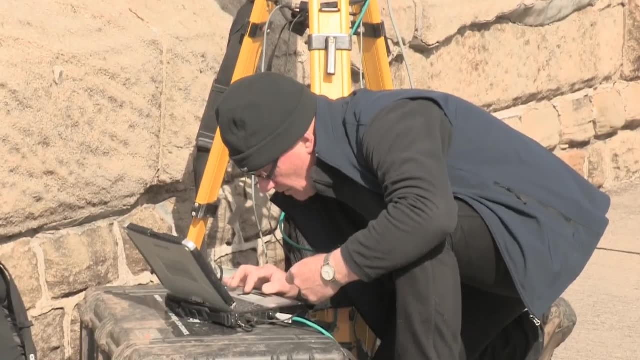 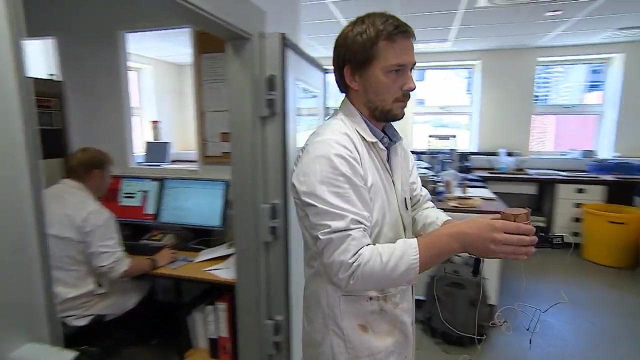 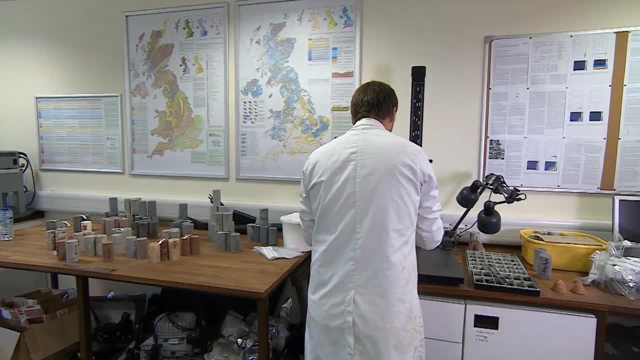 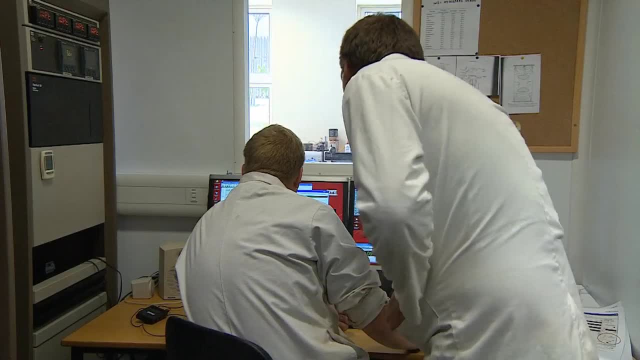 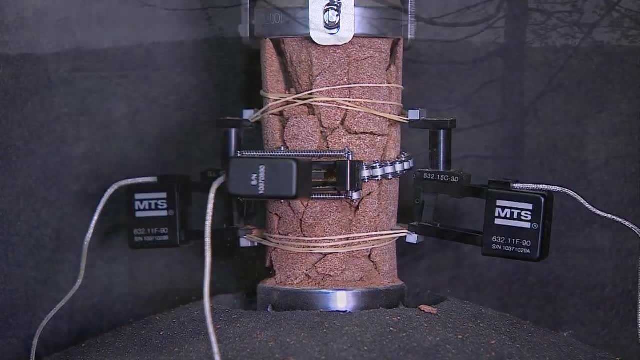 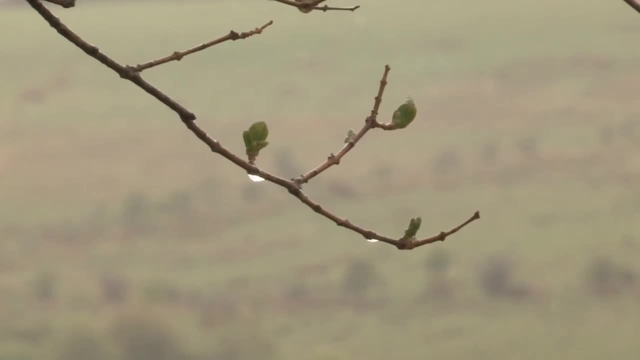 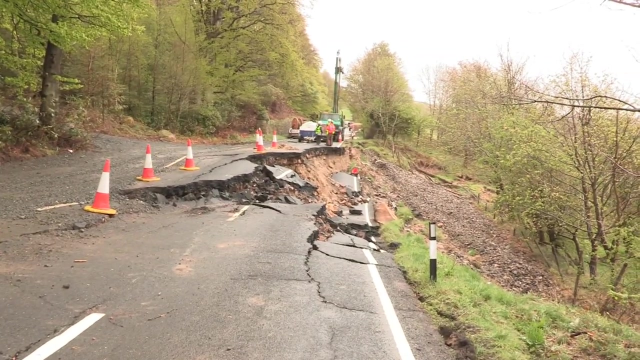 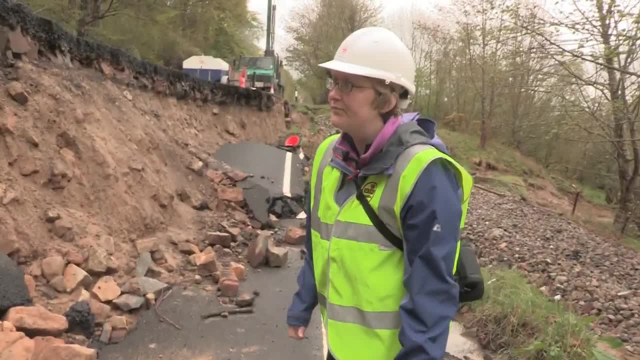 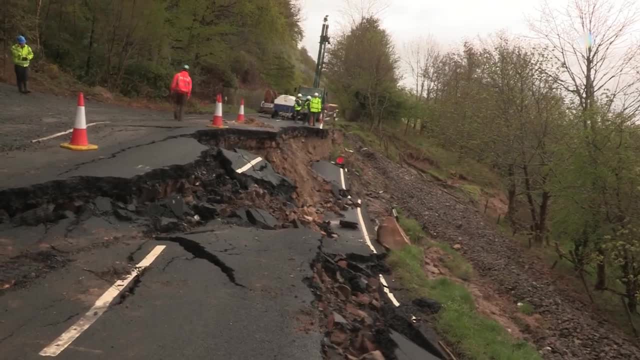 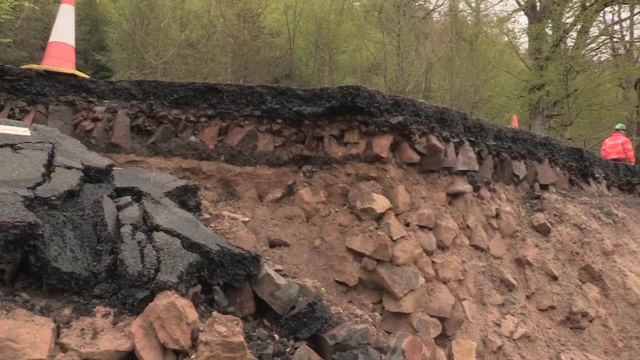 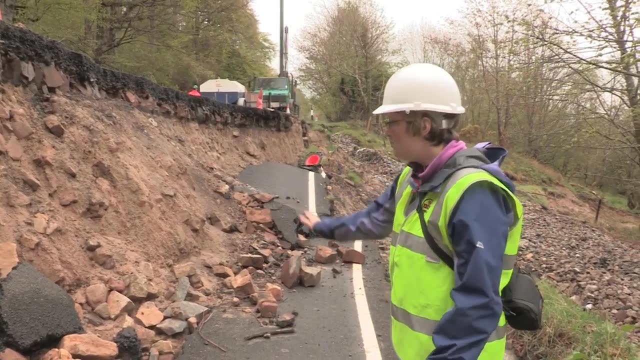 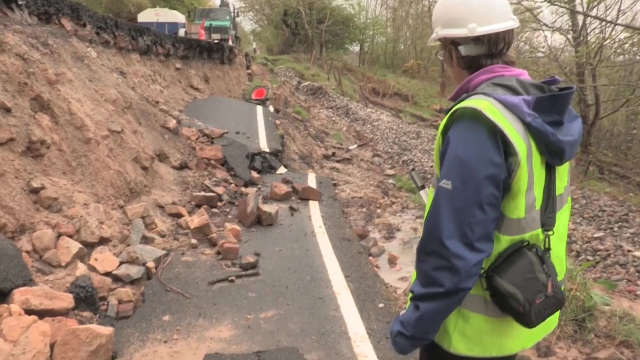 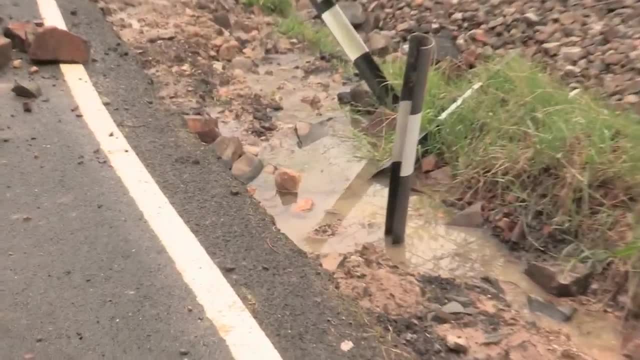 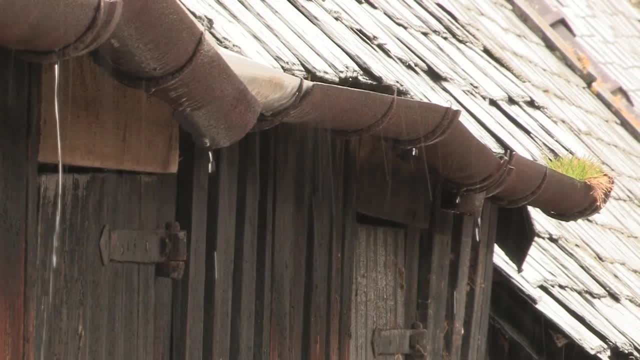 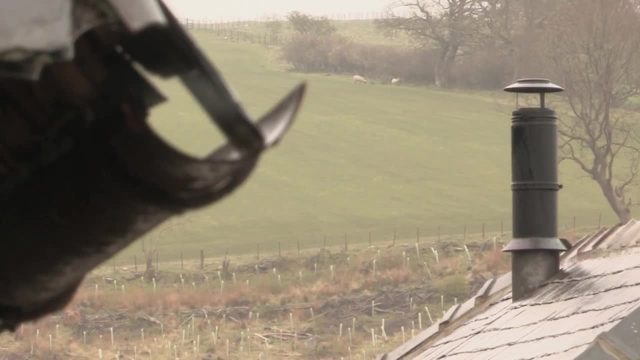 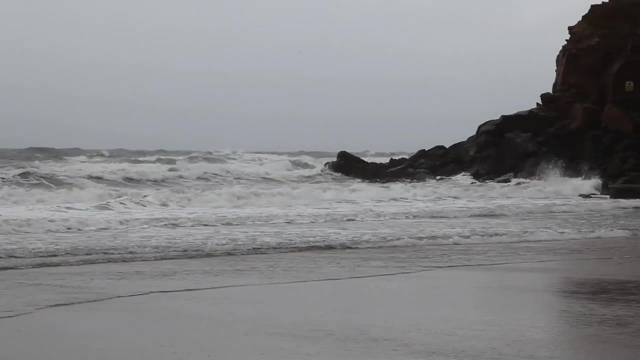 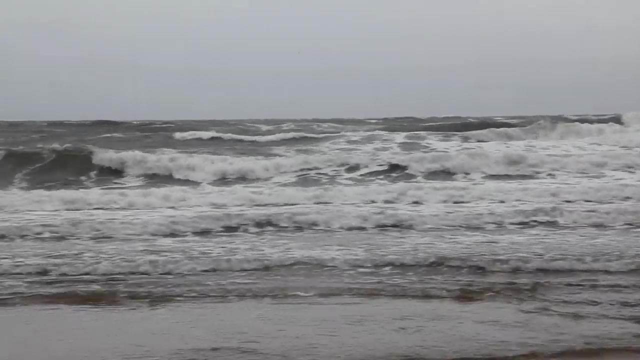 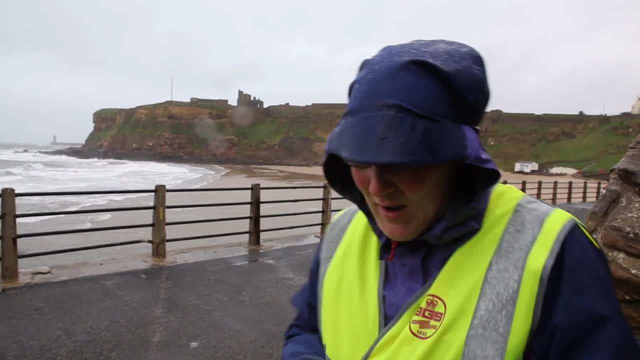 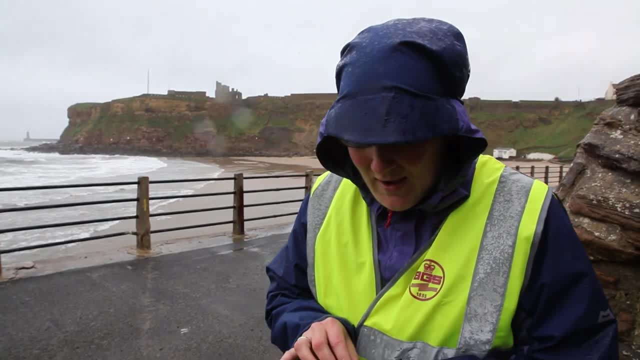 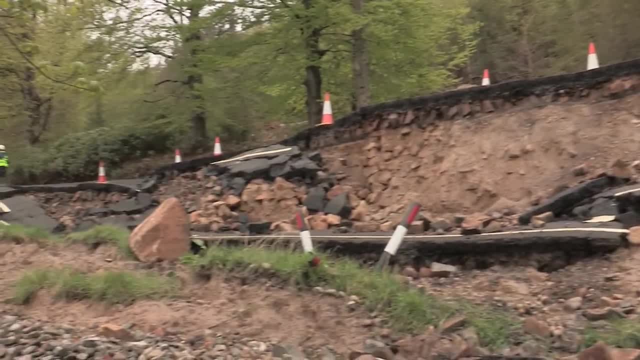 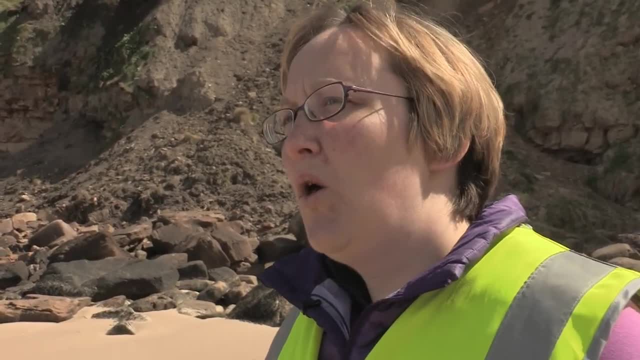 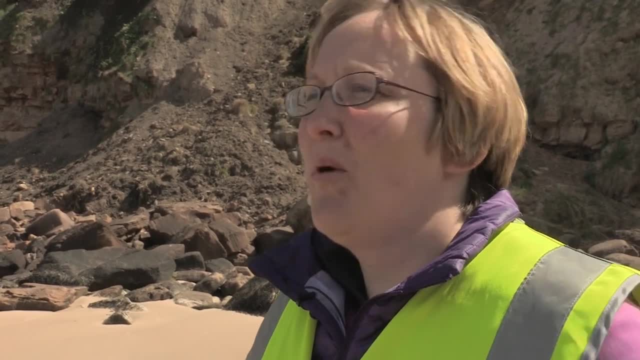 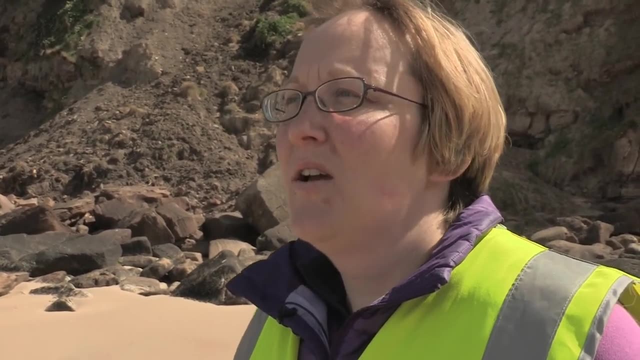 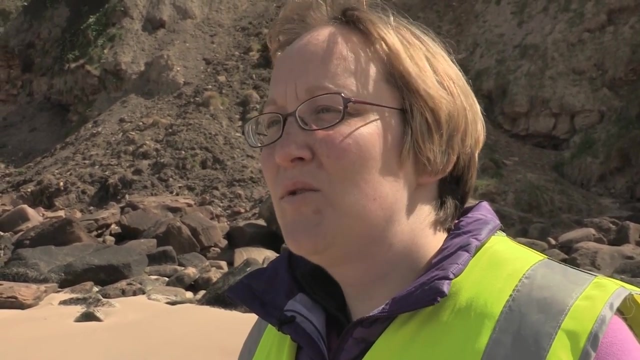 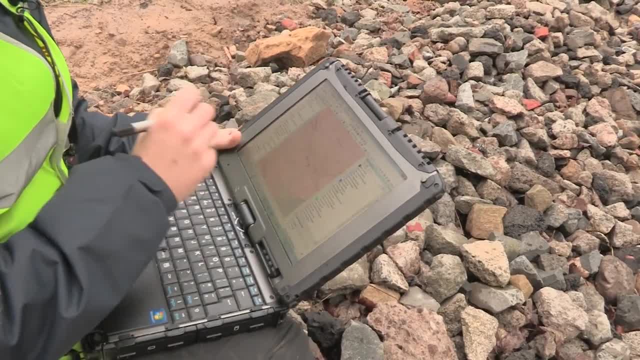 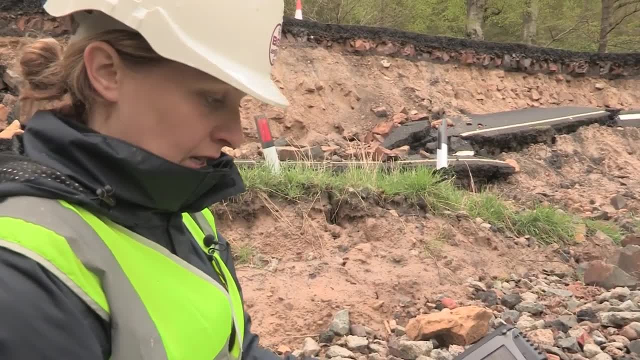 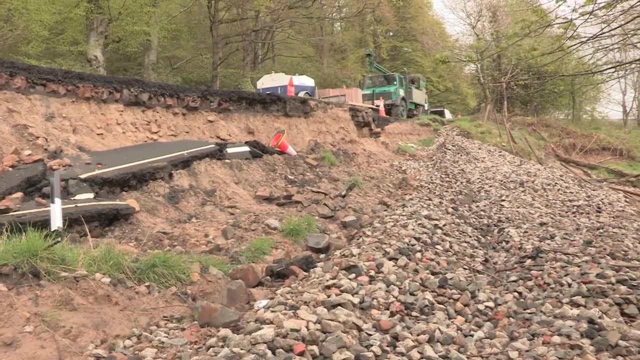 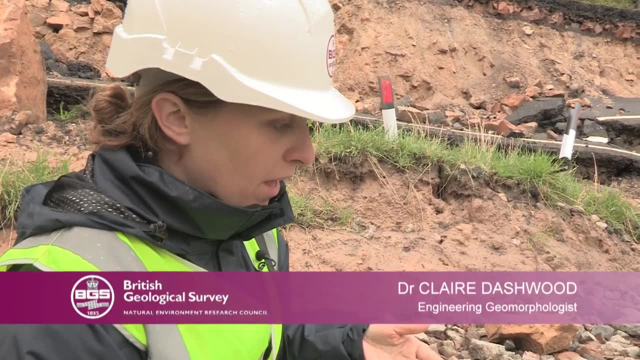 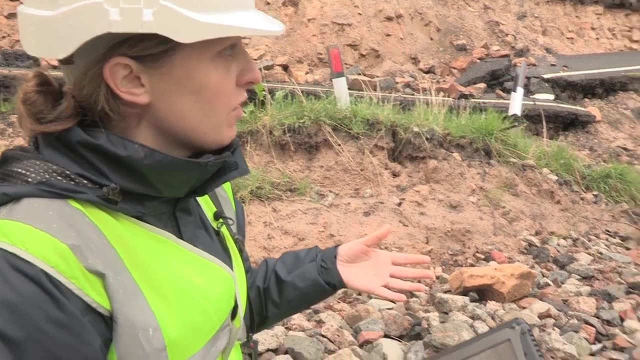 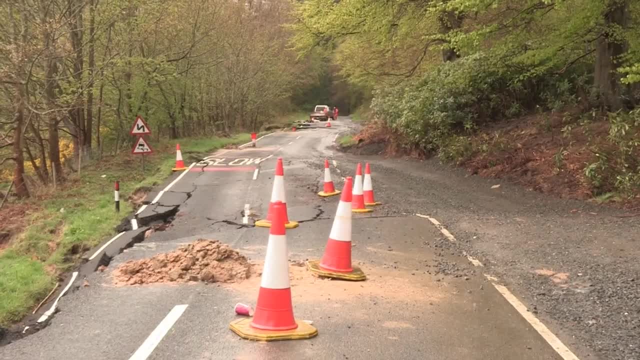 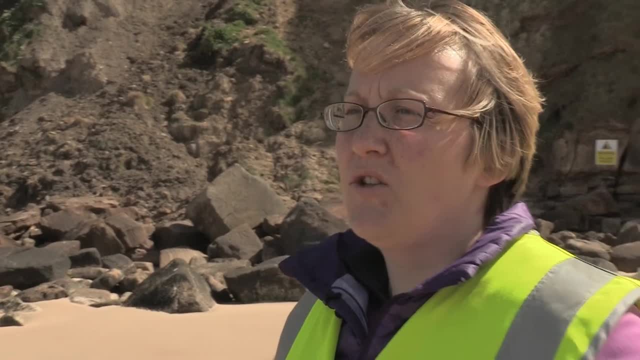 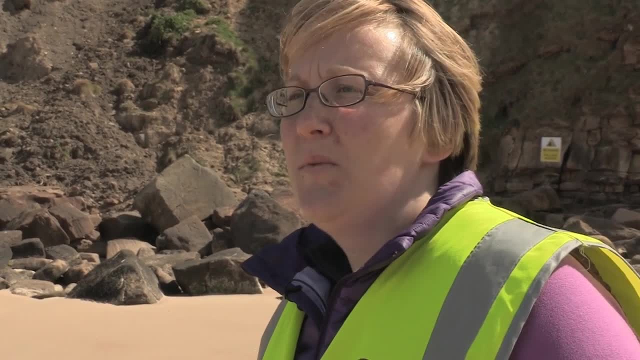 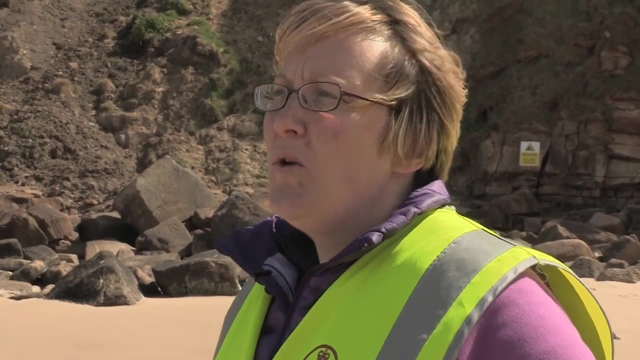 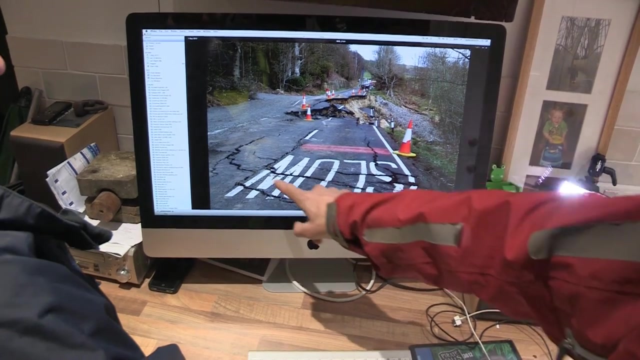 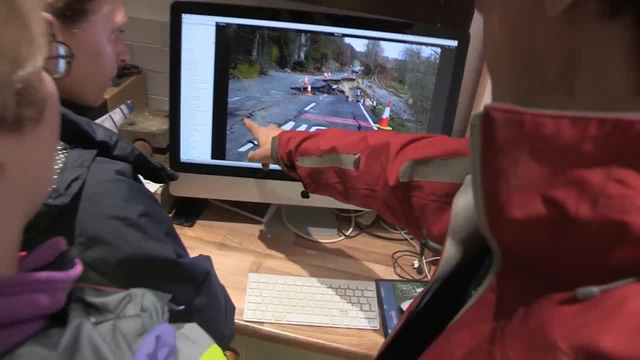 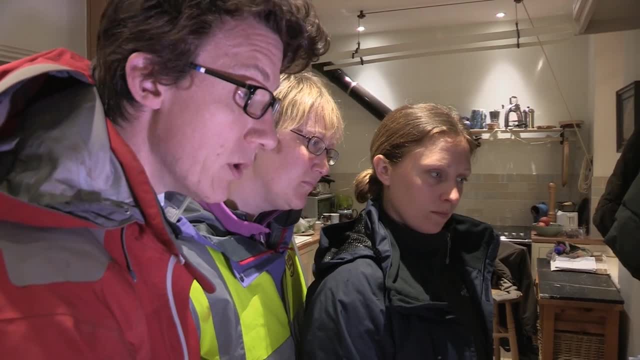 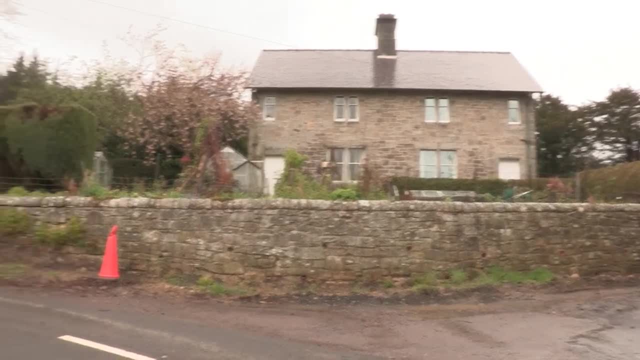 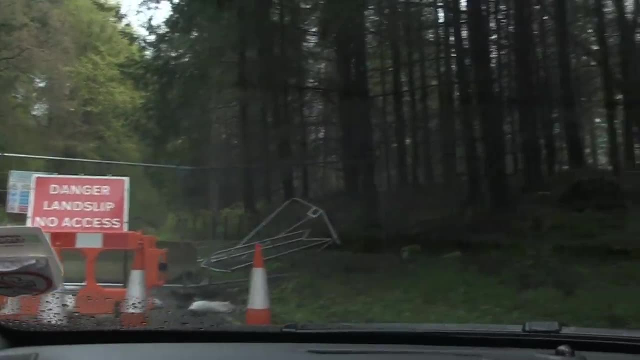 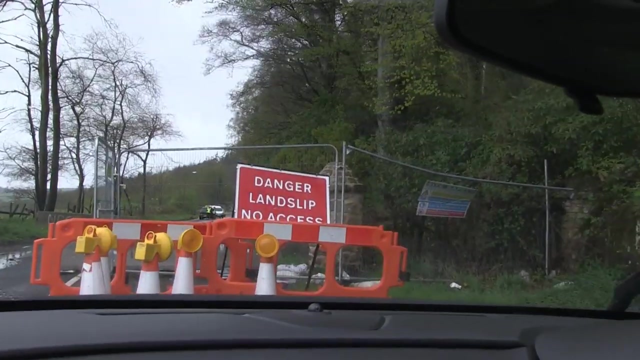 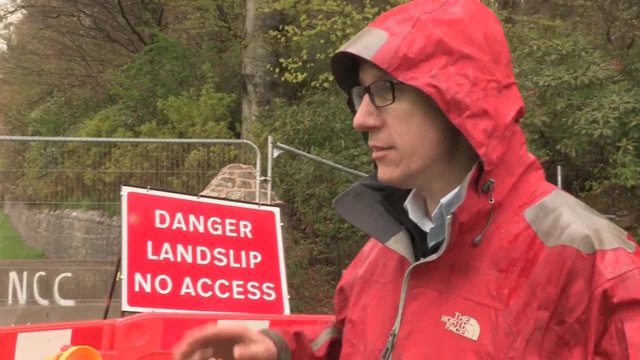 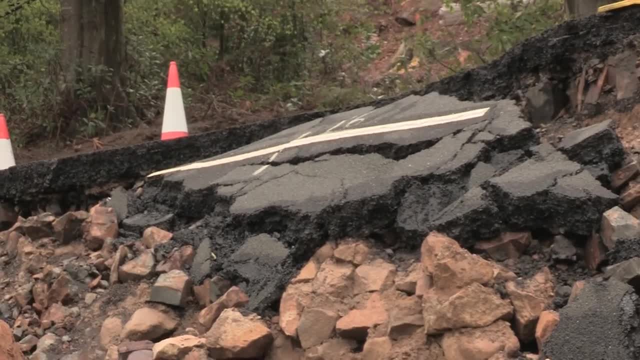 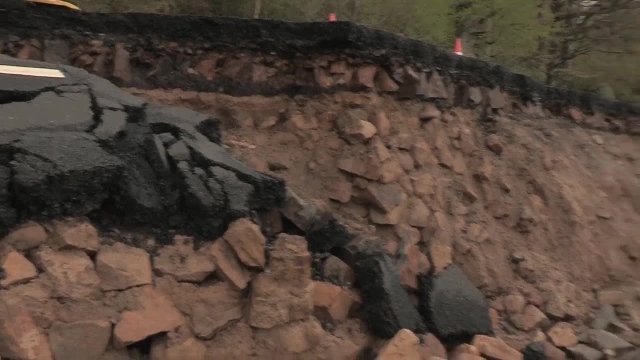 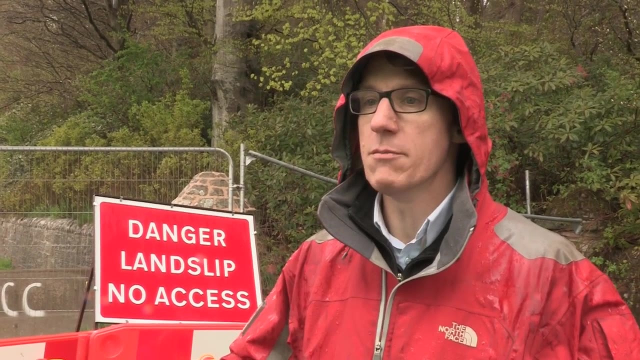 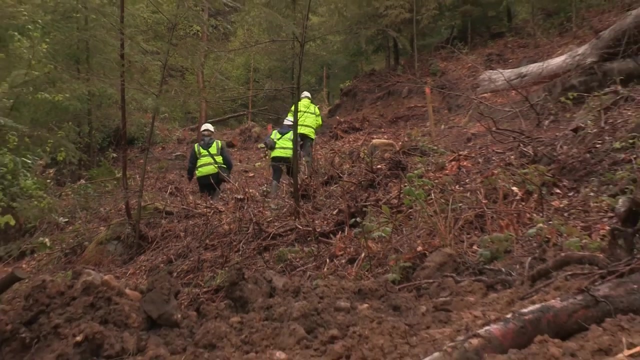 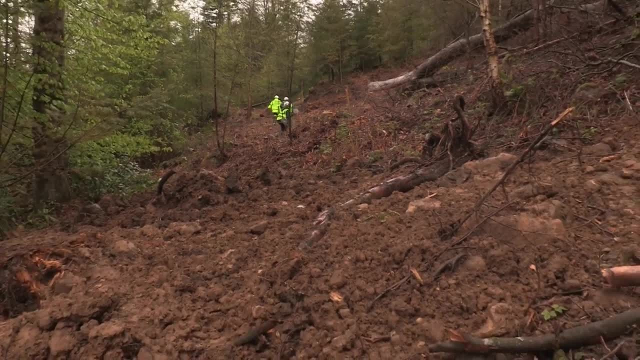 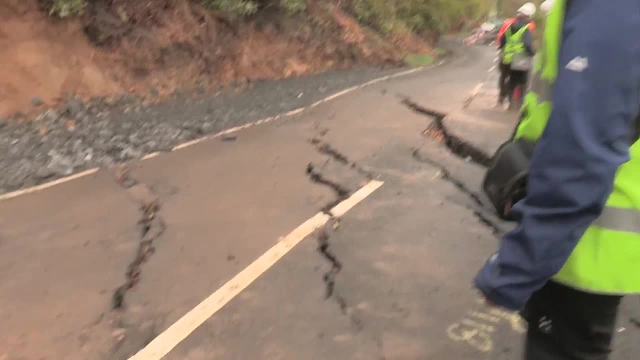 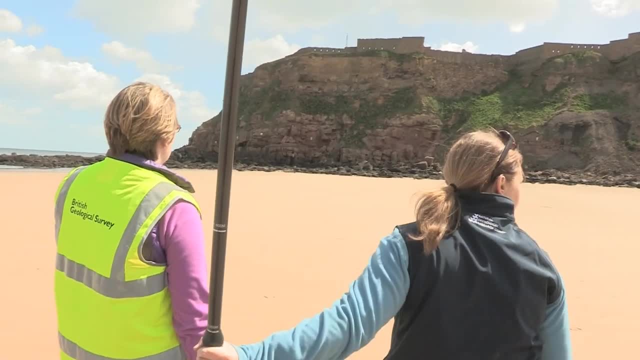 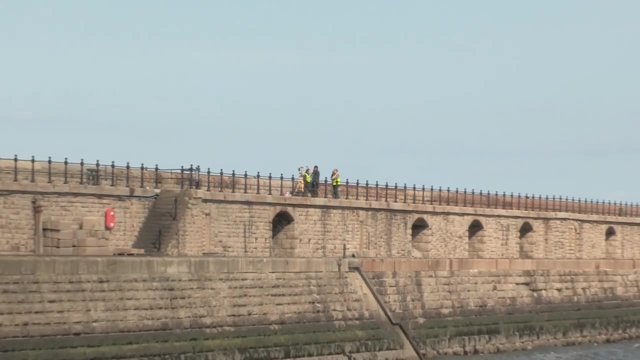 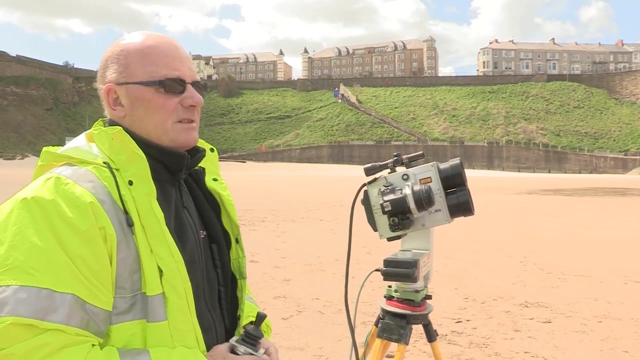 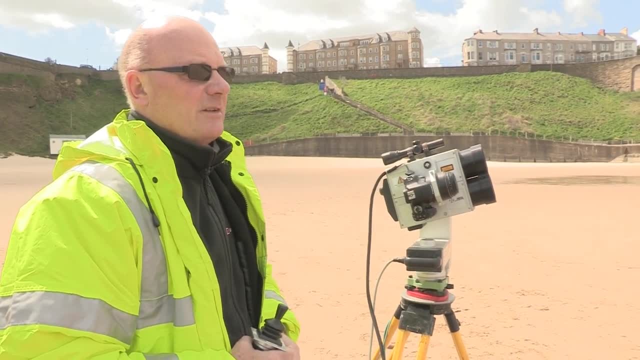 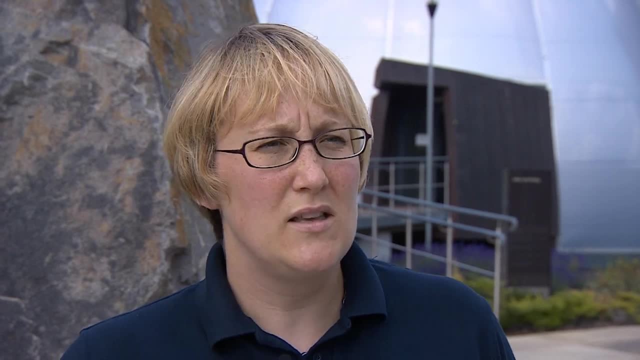 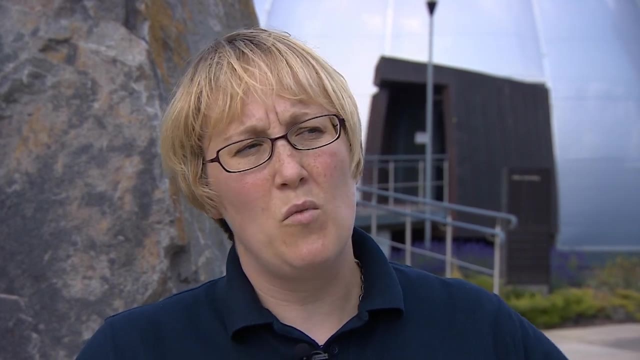 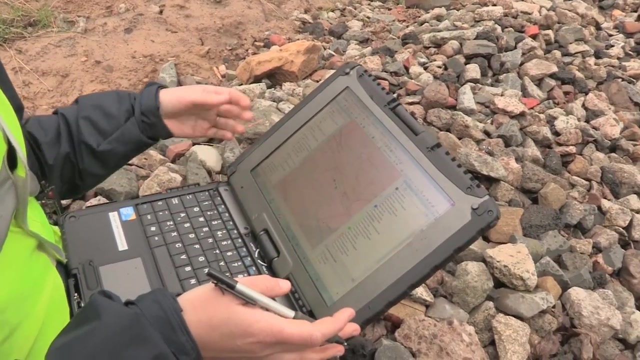 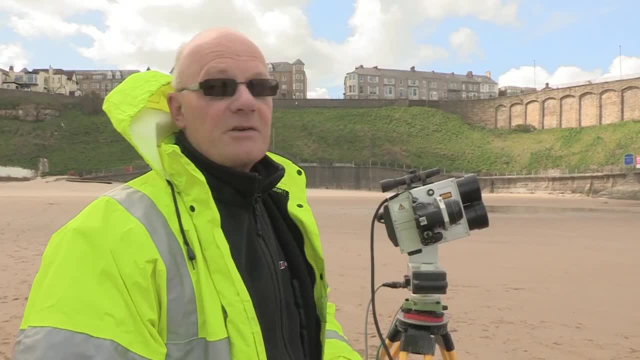 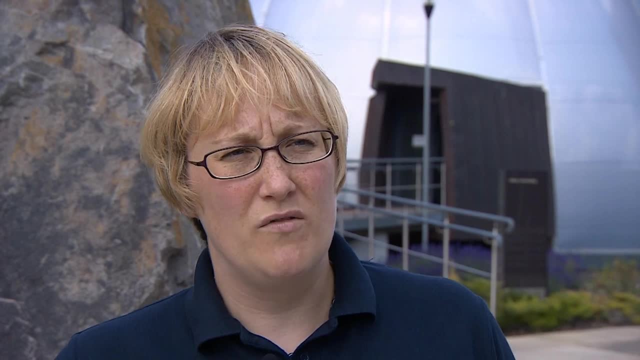 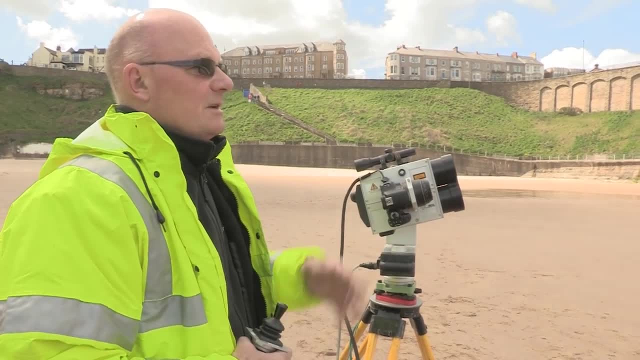 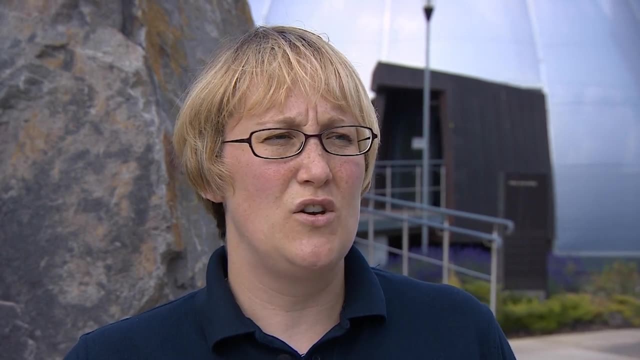 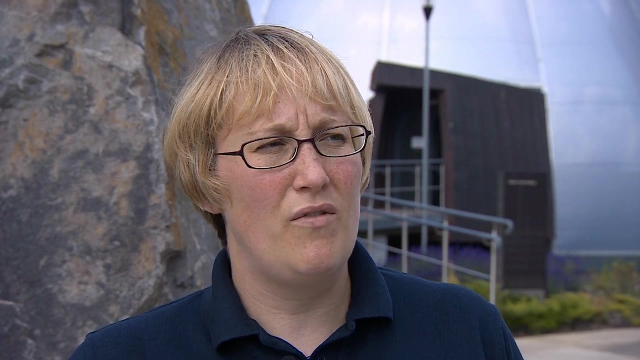 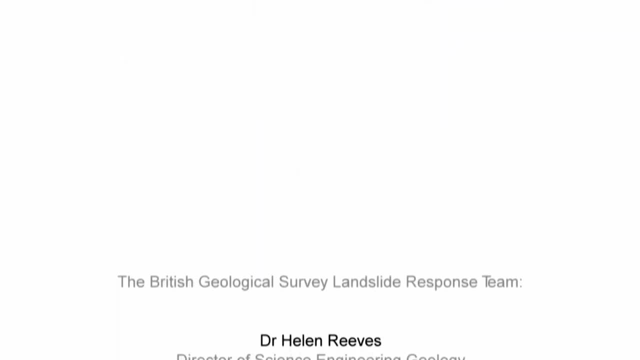 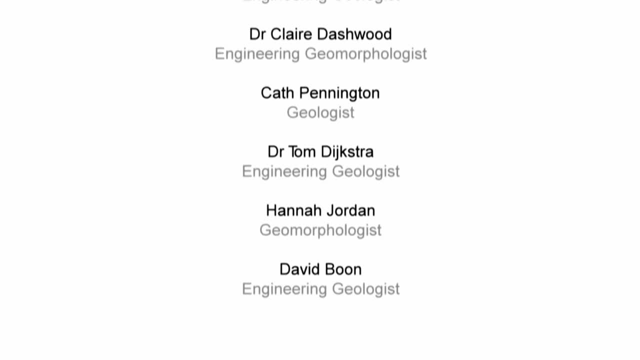 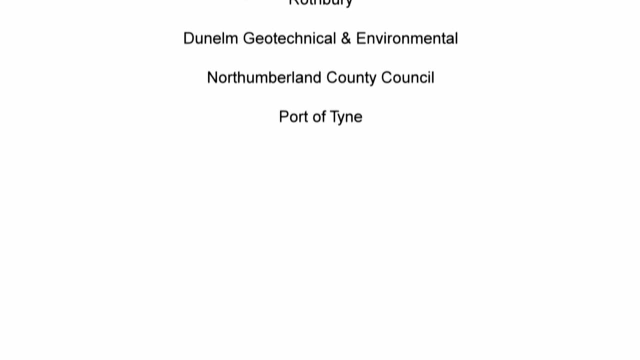